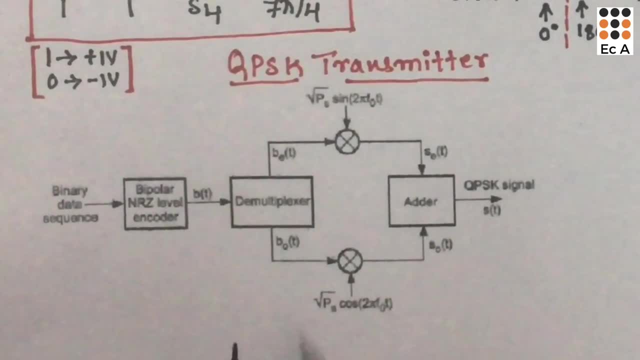 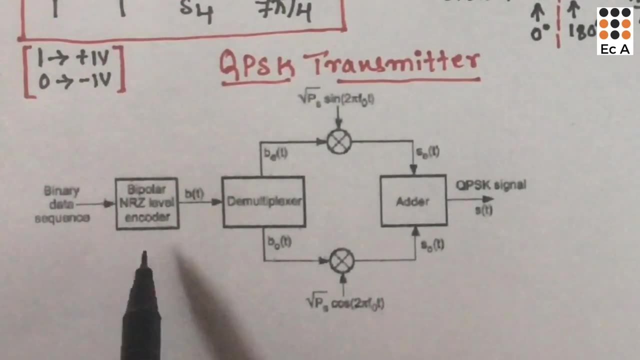 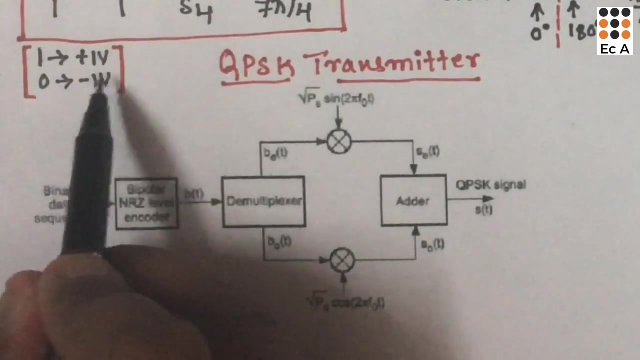 Figure shows the block diagram of QPSK transmitter. The input binary sequence is first converted into bipolar NRZ type of signal. This signal is called as B of T. It represents binary 1 by positive 1 volt And 0 by negative 1 volt. 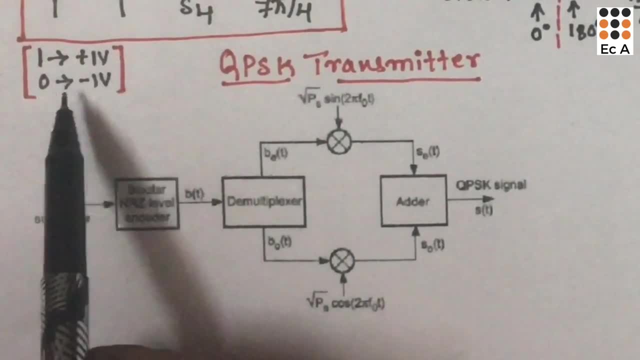 So NRZ signal represents 1 by positive 1 volt, 0 by negative 1 volt. This signal, B of T, is given as input to the demultiplexer. The demultiplexer divides B of T into two separate bit streams. 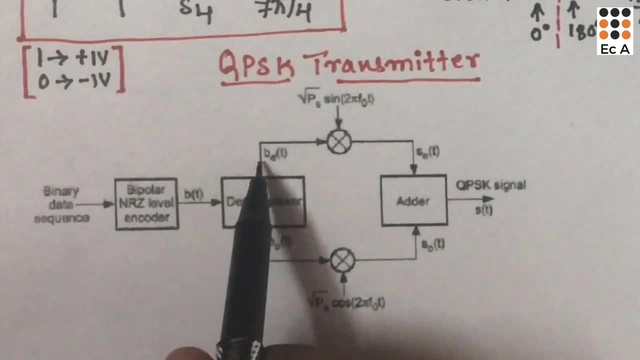 It will divide the signal B of T into even number of bits and odd number of bits. Even number of bits is represented by B E of T. odd number of bits is represented by B 0 of T. So B E of T represents even number sequence. B 0 of T represents odd number sequence. 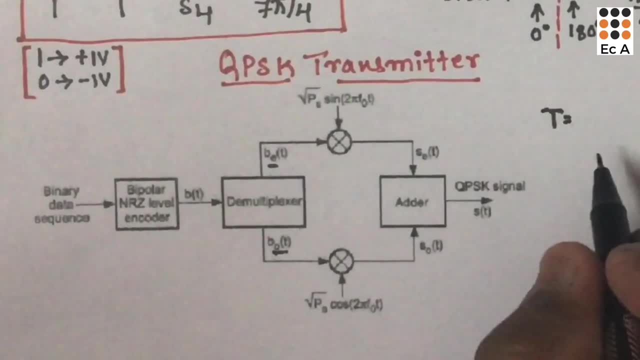 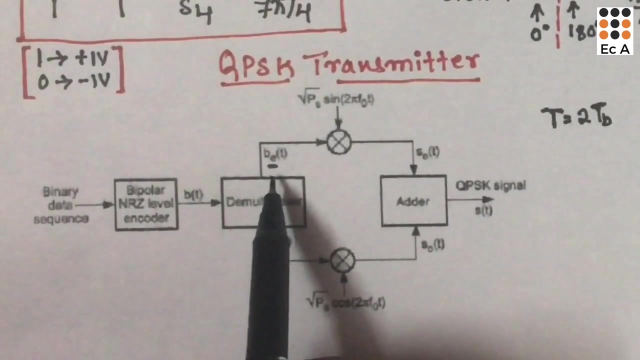 The symbol duration T for both odd and even number sequence will be equal to 2TB. Hence every symbol contains 2 bits. In the triangle we are having two carrier signals. Even bit will be modulated using a carrier signal which is represented by sine wave. 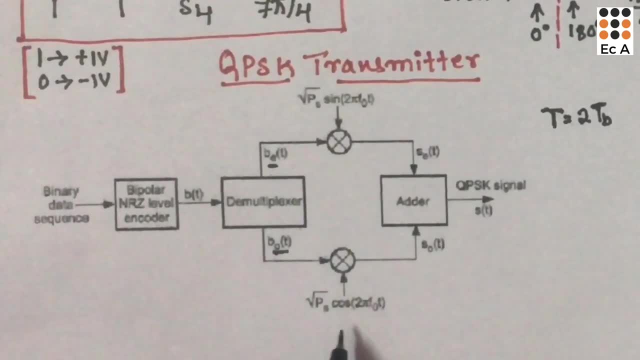 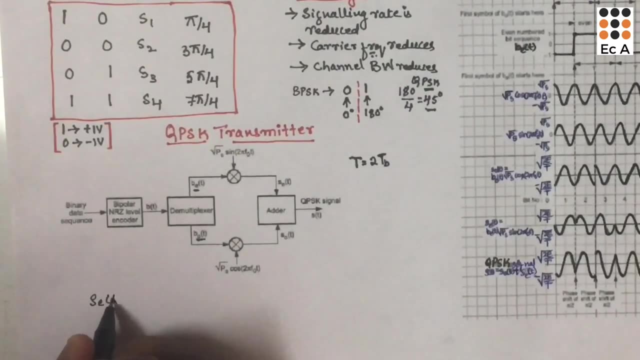 And odd bit- is modulated by the carrier signal, which is represented by cos wave. So we will get two modulated signals that can be represented as: S. E1 of T, which is the even stream, will be equal to B E1 of T, square root of PS. 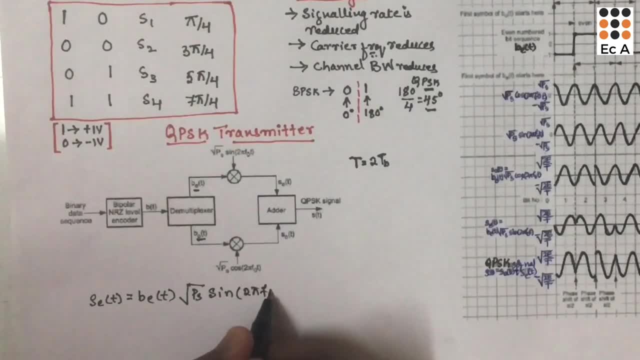 sine 2 pi f0 T and S odd of T is equal to B odd of T, square root of PS, cos 2 pi f0 T. So we will get two sequences: S? E1 of T and S odd of T. The adder adds these two signals and the output of the adder is given as: 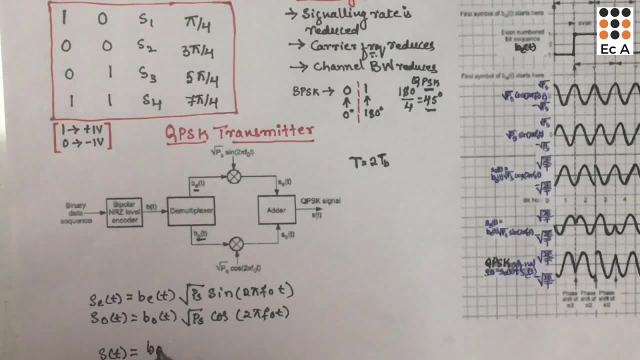 S of T is equal to B 0 of T square root of PS cos 2 pi f0 T, plus B E1 of T square root of PS sine 2 pi f0 T. This equation represents the QPSK signal. Now let us understand the operation of QPSK modulation. 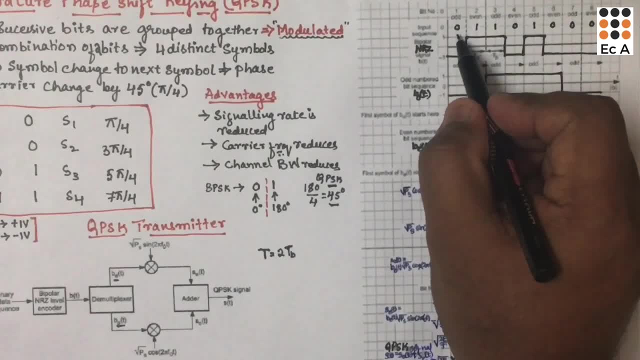 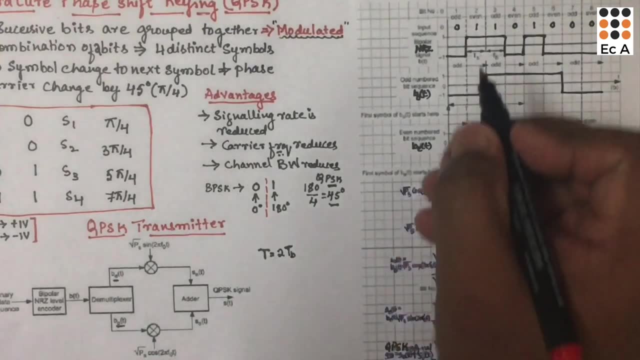 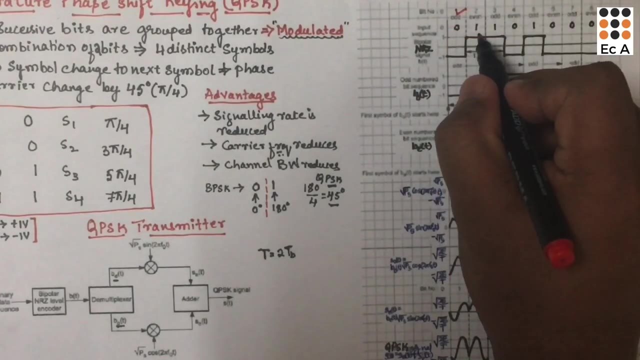 Let us consider the input bit stream: 0 1 1 0. 1 0 0 0.. First let us identify the even bits and odd bits in this sequence. So in the input sequence the first bit is the odd bit, next you will get the even bit. 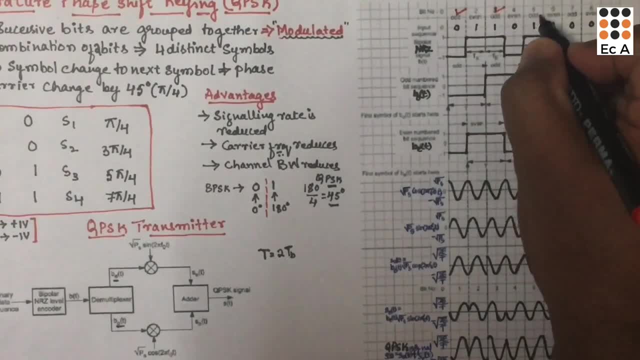 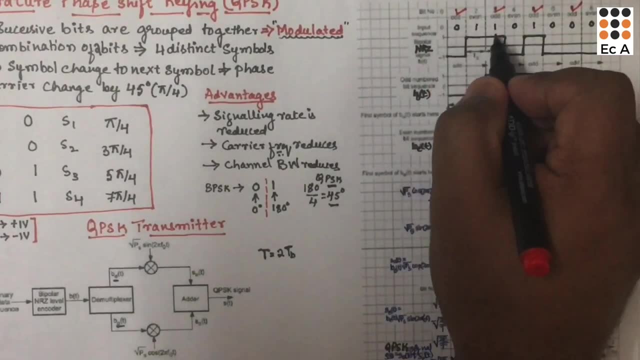 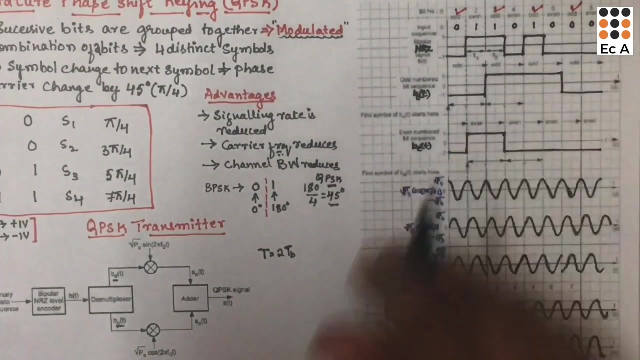 after that you will get the odd bit, then it is even bit, then odd bit, then even and odd bit. So we will get the odd bit as 0, 1.. 1, 0 and the even bit as 1 0, 0, 0.. 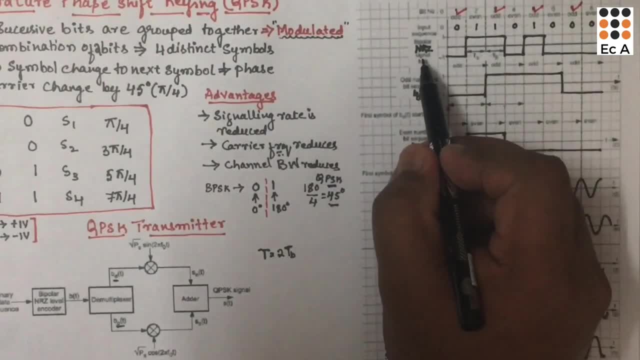 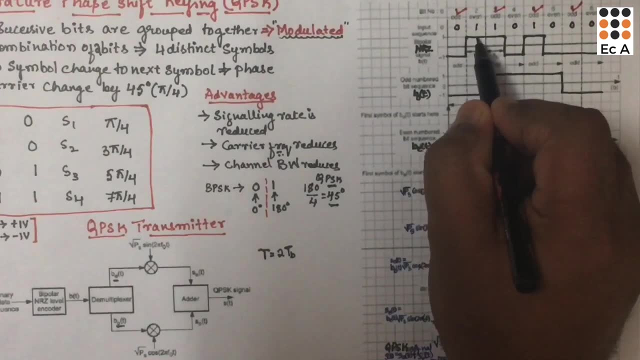 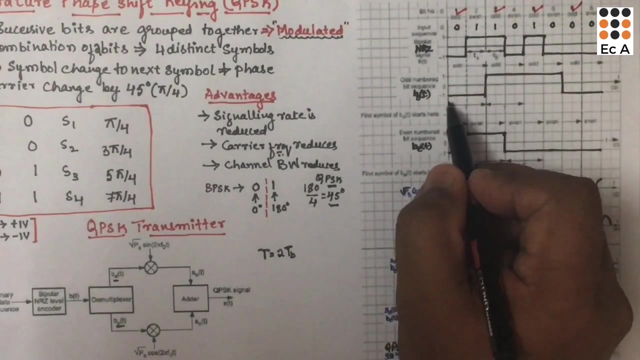 Now let us represent this input sequence in the form of NRZ, which is non-written to 0.. 0 will be represented as minus 1 and 1 will be represented as plus 1 in NRZ encoding. Now we will consider odd bits and we will represent it as an odd sequence. 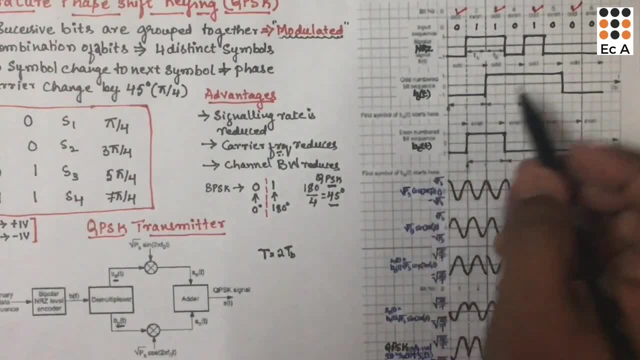 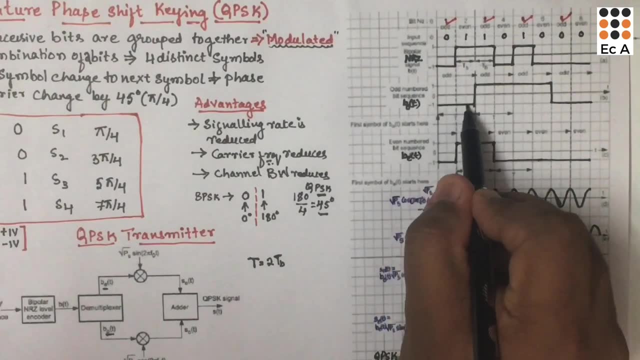 Time duration of each bit will be 2 bit Period. So we have the odd sequence 0, 1, 1, 0.. So 0 is represented for 2 bit period, Then 1 is represented for 2 bit period. 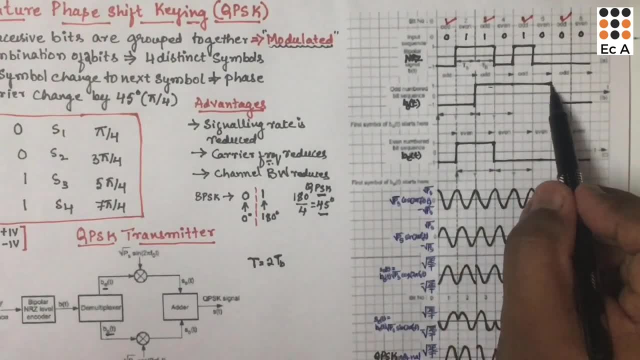 Again, 1 is represented for 2 bit period and 0 is represented for 2 bit period. In the same way we will represent the even bits as an even number sequence. So if you observe here, the even bit will start after the odd bit. 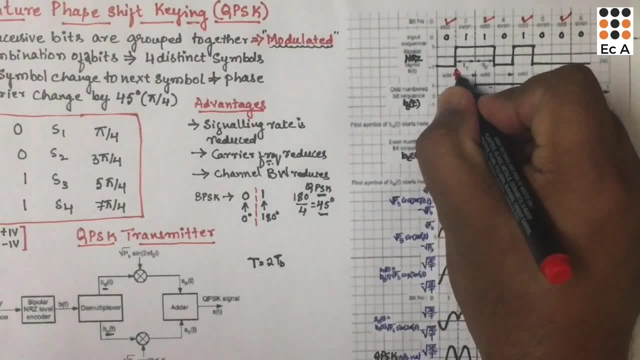 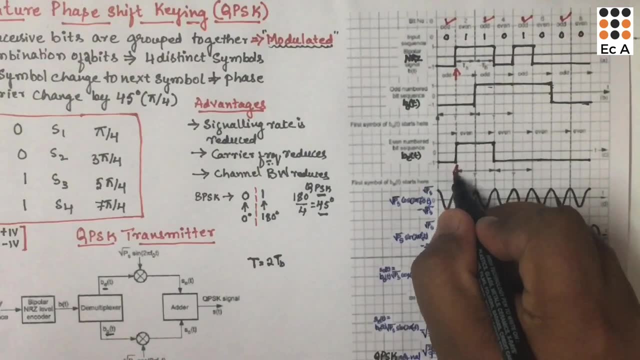 and it will commence from this position. So from this position the even bit will start. So that is why, while representing the even sequence also, we will start with this position And before that position we will write it as 0.. 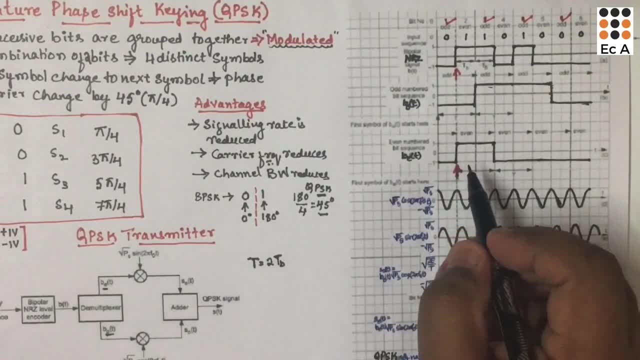 So after 1 bit delay, the even bit sequence will be represented. So the even bit sequence is 1 0 0 0.. Now we will start representing the even sequence from this position. 1 will be represented for 2 bit period. 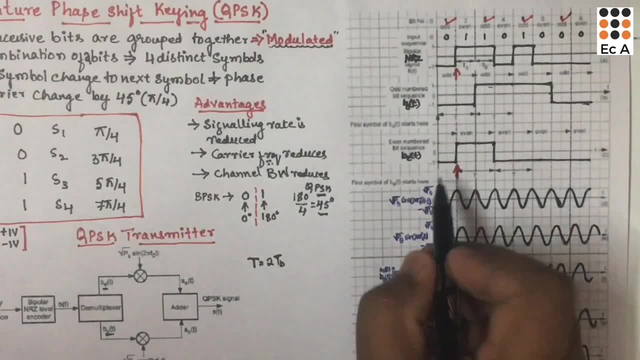 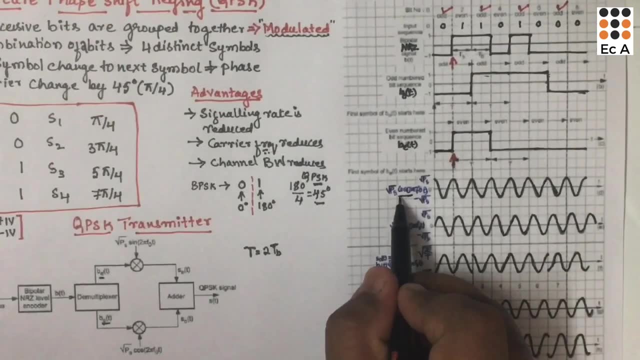 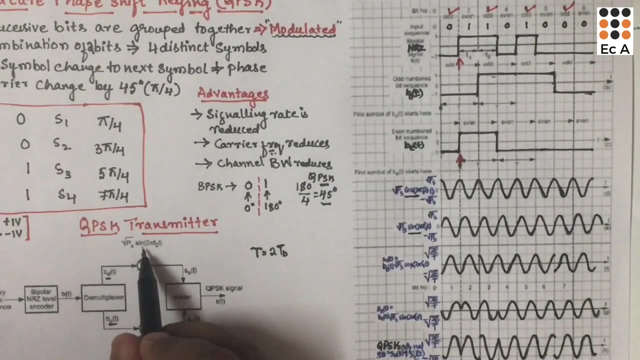 Then it is 0 0 0. So before this position we will take it as 0.. Now we will take 2 carriers. First carrier is represented by cos and the second carrier is represented by sin. Even bit will be modulated using sin wave. 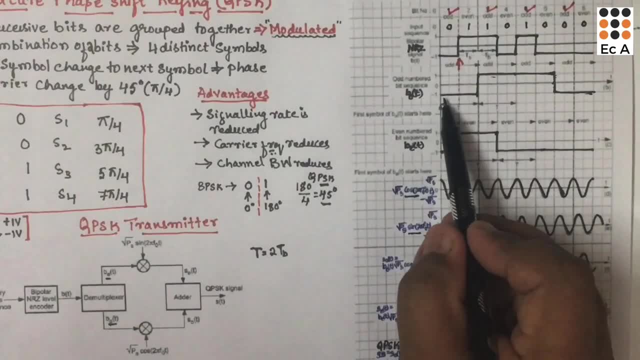 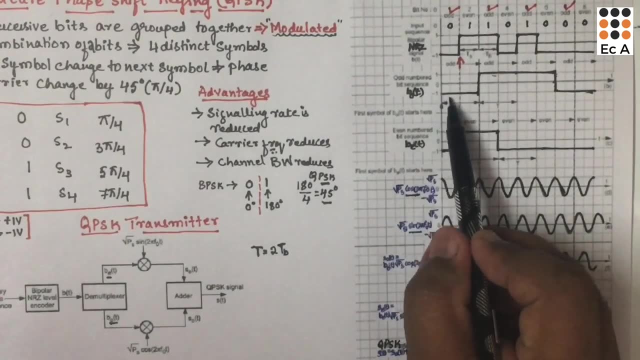 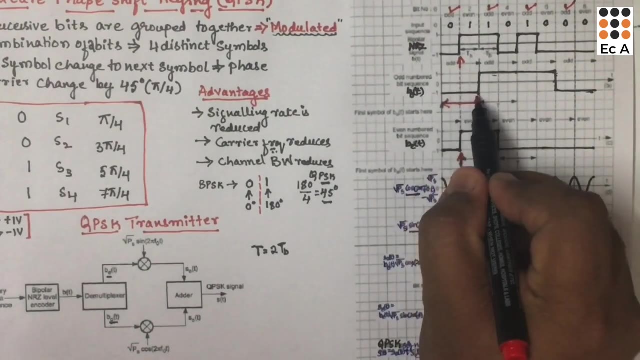 Odd bit will be modulated using cos wave. Now let us take the odd bit and the cos wave and modulate the cos wave. Now, if you take the odd bit up to this position, you are having 0, which means the value of the odd sequence is minus 1.. 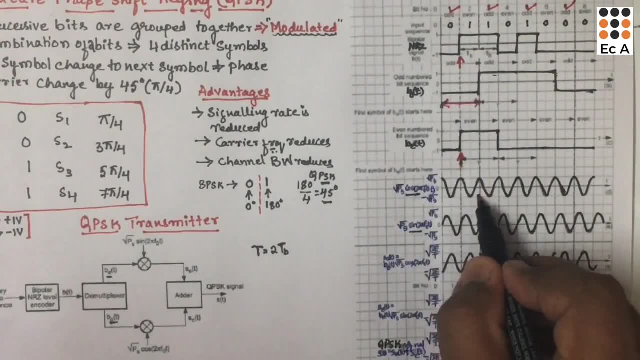 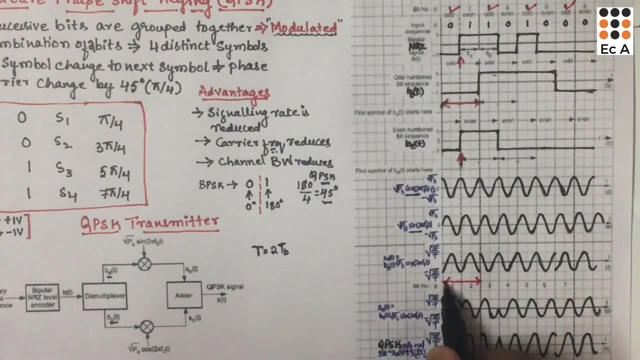 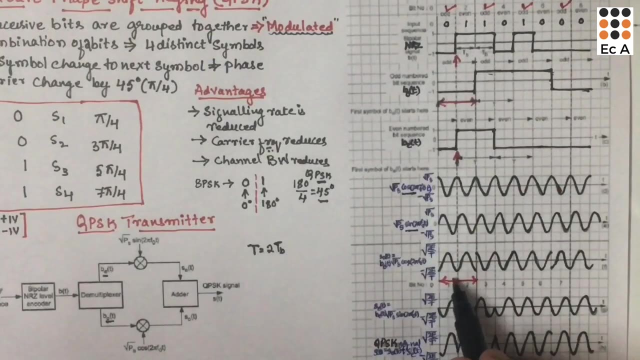 This minus 1 will be multiplied with cos signal and you will get a cos wave which will be inverted here, which will be having a phase shift, Since it is minus 1 multiplied with cos signal. so minus 1 will change the phase of the carrier. 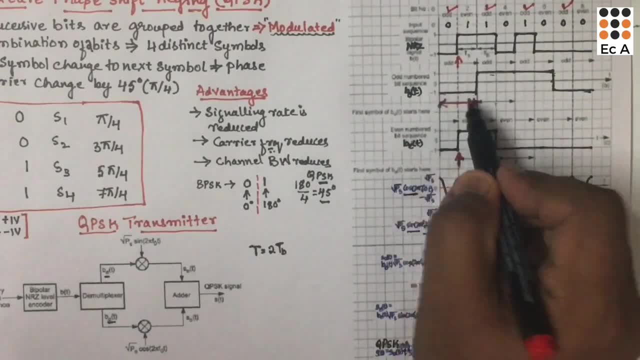 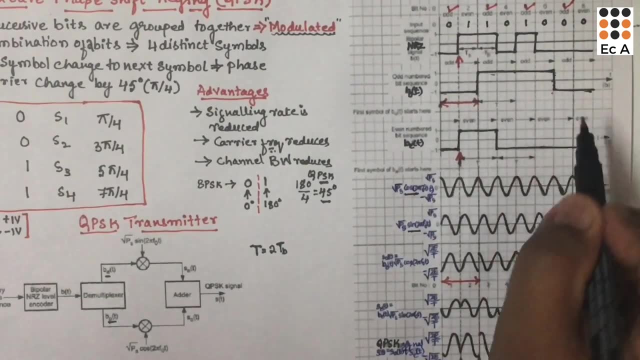 So that's why, for this time period where you are having minus 1, the cos wave will change its phase. So from this point to this point, you are having plus 1 and the cos wave, up to this point, will not change. 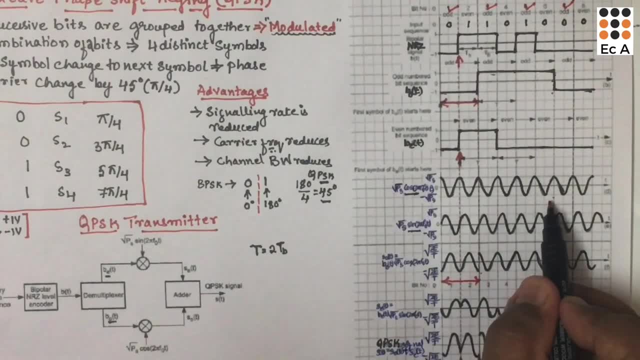 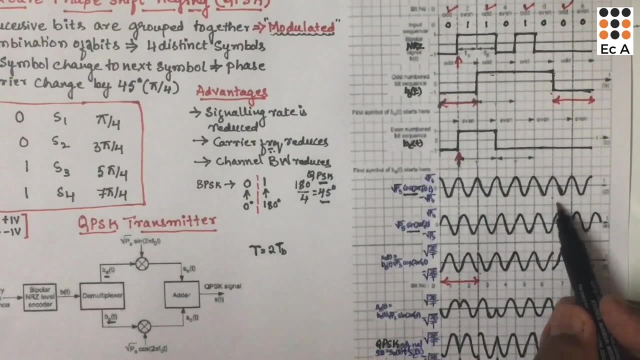 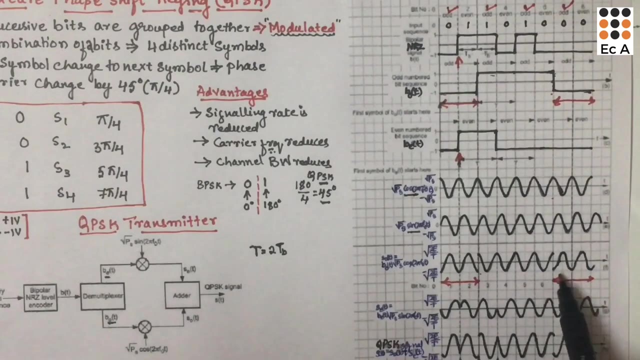 You can see, it is same as the cos wave which is transmitted here, And here again you are having a phase shift of minus 1.. So the cos wave will change its phase for this position. So since minus 1 multiplied with cos wave, you will be having a phase shift here. 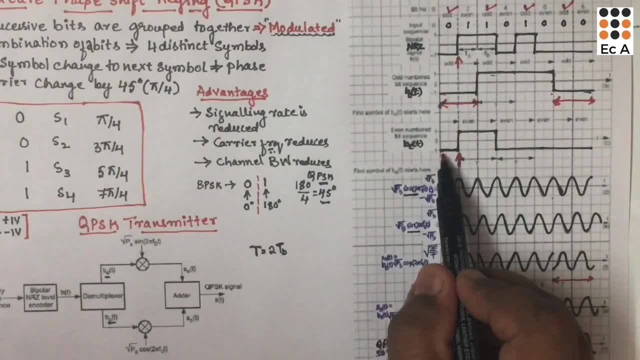 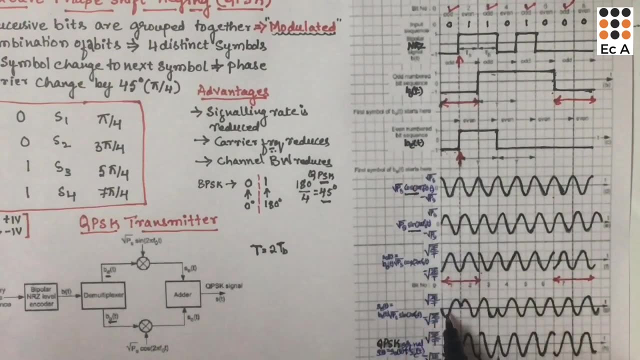 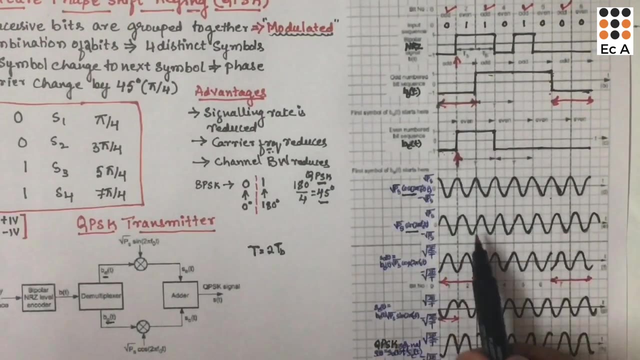 Now in the same way for even bits. here you are having minus 1 up to this point. Minus 1 multiplied with sine wave, you will be having a phase shift here. And 1 multiplied with sine wave, you will get the actual sine wave. up to this point. 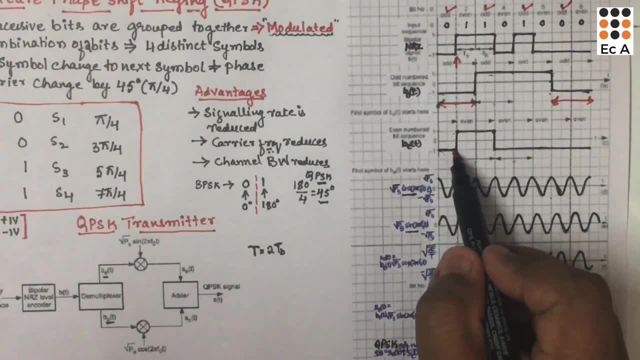 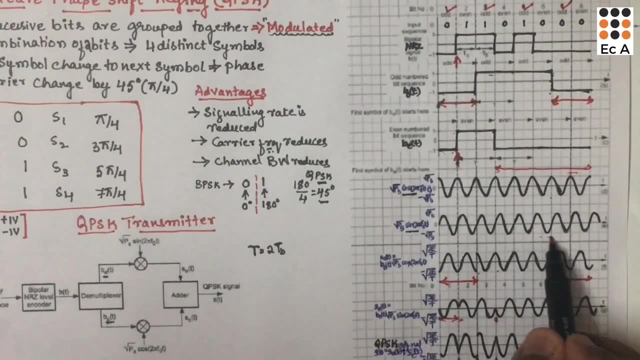 So from here to here you will get a sine wave as it is, because you are having 1 here. After this you are having minus 1, which is multiplied with sine wave up to this point. So you will be having a phase change of sine wave from this point to this point. 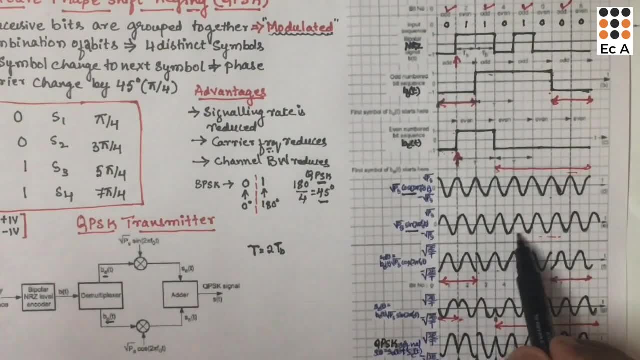 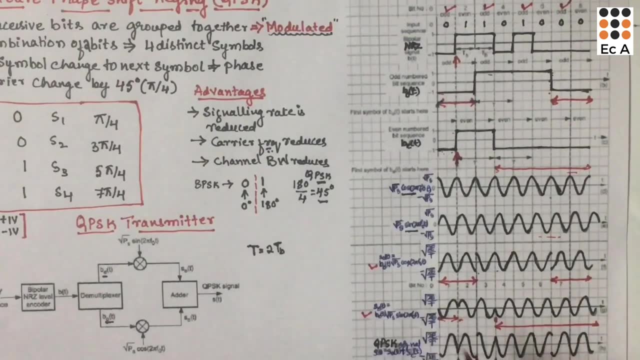 because you are multiplying with minus 1 with a sine wave you will get a phase change. Now we got two signals, odd signal as well as even signal. So these two signals should be added to get a QPSK signal. 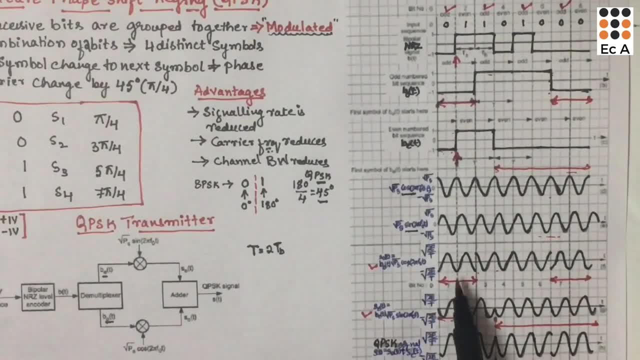 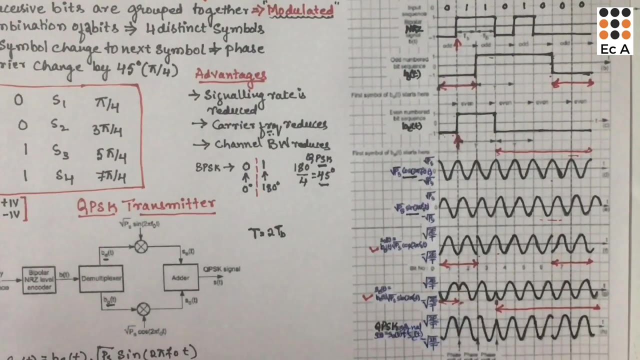 So this is the QPSK signal which is obtained after addition of these two signals, And you can observe there is a phase change in the output when there is a phase change at the input as well. So this is the output of QPSK signal after adding these two signals. 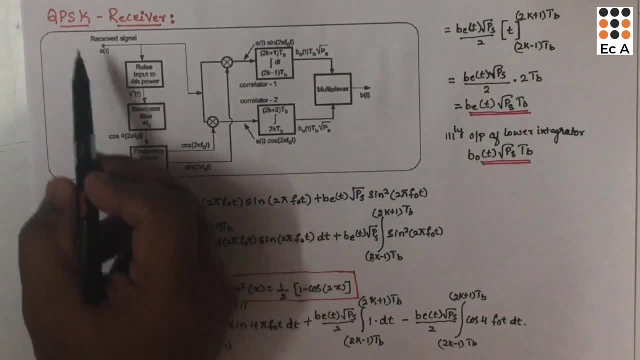 This is about the QPSK transmitter. Now let us understand QPSK receiver. This figure shows the QPSK receiver. Here the received signal S of t, is first raised to fourth power. So the output of this will be S to the power of 4 t. 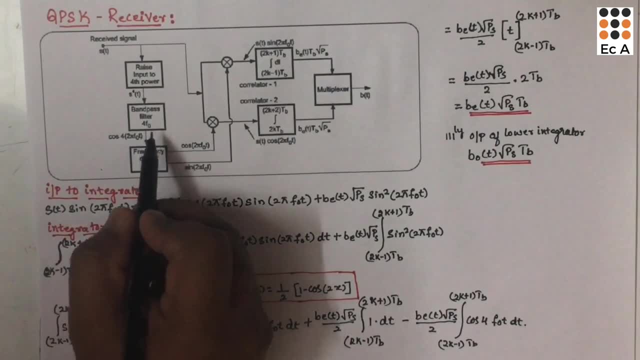 This is passed through a band pass filter centered across 4 f0.. The output of the band pass filter is the coherent carrier of frequency 4 f0.. So we will get the output as cos 4 of 2 pi f0, t. 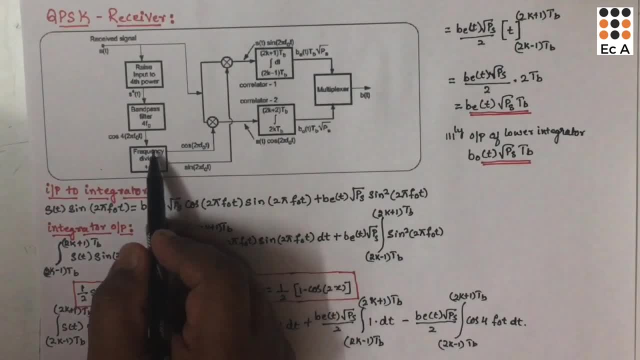 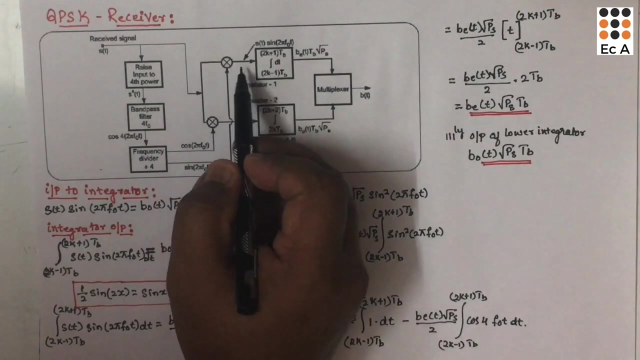 This signal is divided by 4 using a frequency divider. The output of frequency divider will be two carrier signal: cos 2 pi f0 t and sine 2 pi f0 t. These two carriers are applied to two synchronous demodulators. These synchronous demodulators consist of multiplier as well as integrator. 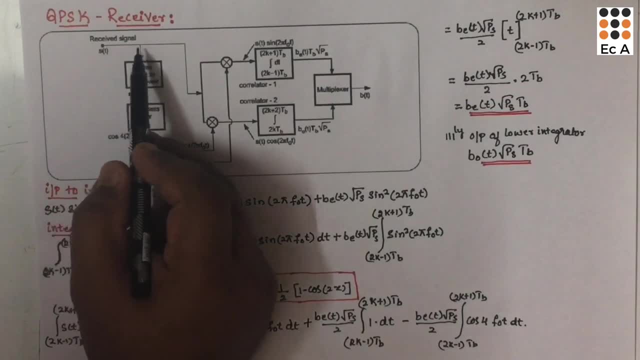 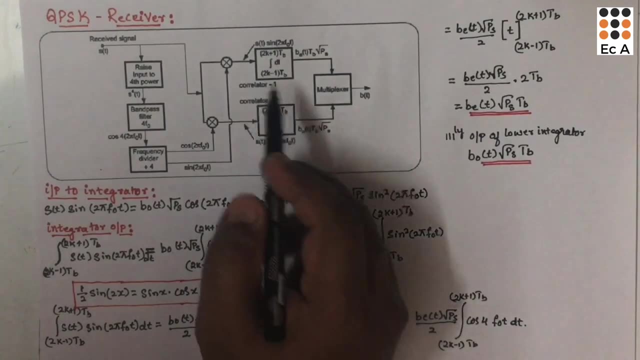 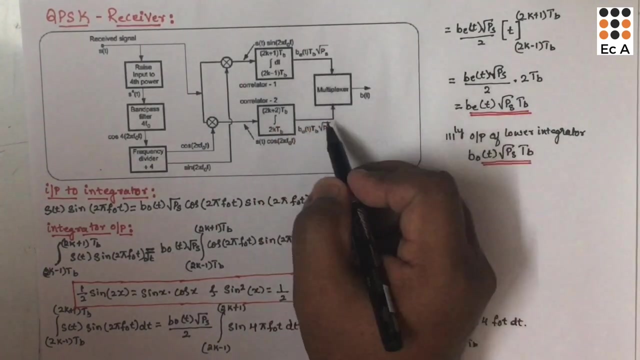 Along with these two carrier signal. the incoming signal is applied to both multiplier. The integrator integrates the product of these two signal over 2 bit period. At the end of the period the output of integrator is given as input to the multiplexer and multiplexer will give the output signal b of t. 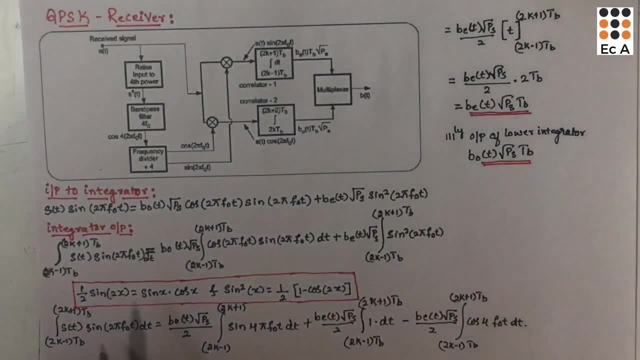 Now let us understand how the integrator works. To the integrator, the input signal applied is S of t into sine 2 pi f0 t. S of t is the received signal. This is the carrier signal, So it will be b0 of t root ps, cos 2 pi f0 t sine 2 pi f0 t, plus b even of t root ps sine square 2 pi f0 t. 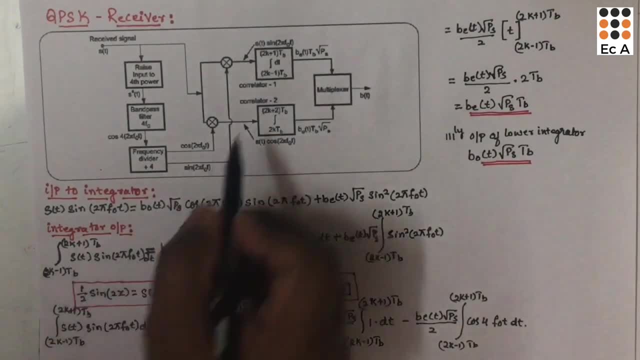 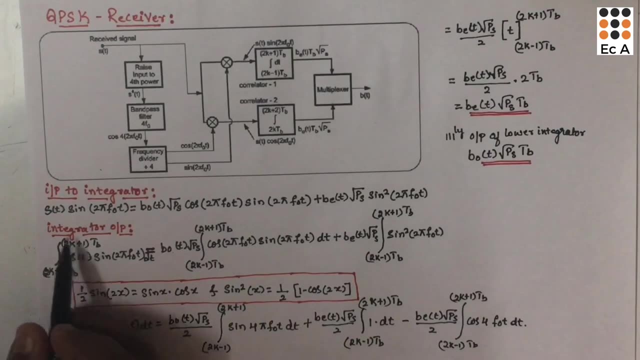 Now the output of the integrator will be between the limits 2k minus 1 tb To 2k plus 1 tb, because we need to consider 2 bit period. So it will be integration between the limits S of t. sine 2 pi f0 t dt will be equal to b0 of t. integration of 2k minus 1 tb up to 2k plus 1 tb, cos 2 pi f0 t into sine 2 pi f0 t dt. 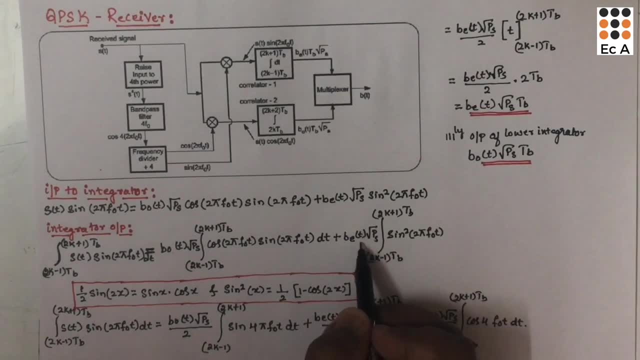 So we have written this b0 of t plus b, even of t root ps, integration of 2k minus 1 tb up to 2k plus 1 tb. sine square 2, pi, f0, t. Now we can use the formula 1 by 2. sine 2 x can be given as sine x into cos x and sine square x. 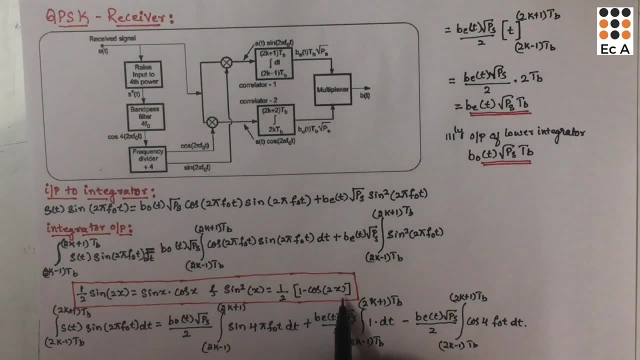 We can write it as 1 by 2, 1 minus cos 2 x. Using this formula, we can write the above equation: as we will be having the left hand side In the top right-hand side, it will be b0 of t root ps divided by2. integration of 2k minus 1 tb up to 2k plus 1 tb sine 4pi, f0, t, dt. 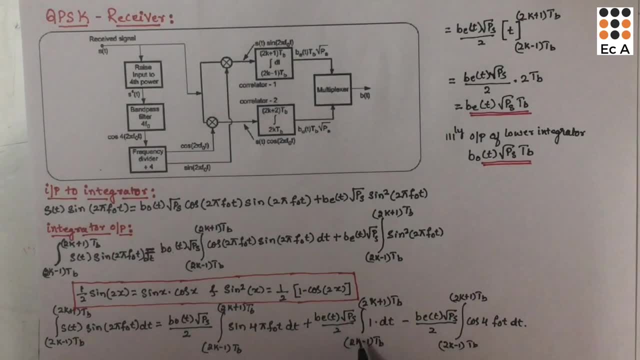 plus b, even of t root ps divided by 2: integration of 2k minus 1 tb up to 2k plus 1 tb. 1 dt minus b1 of t root ps divided by 2: integration of 2k minus 1 tb. 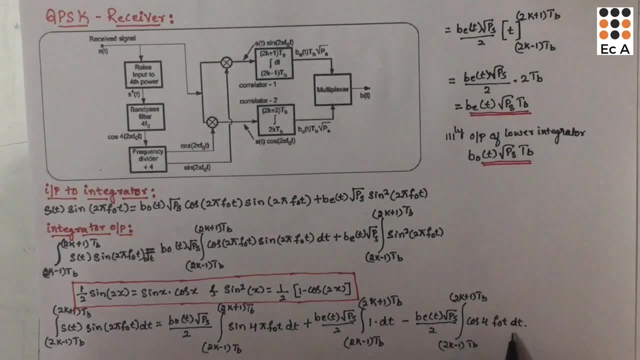 2k plus 1 tb, cos 4, f0, t, dt. In this equation, first and third integration involves the integration of sinusoidal signal over 2 bit period. So integration of sinusoidal signal over 2 bit period will be equal to 0.. So the first and third integration will be equal to 0. So we will be. 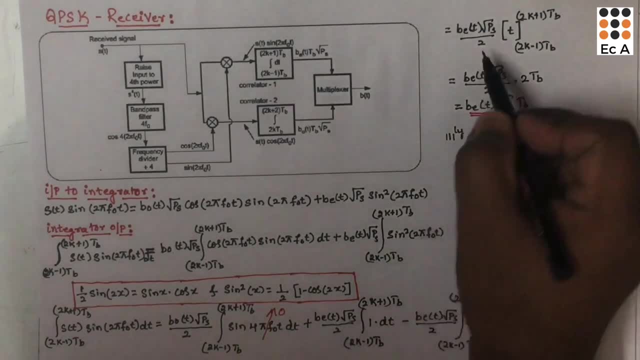 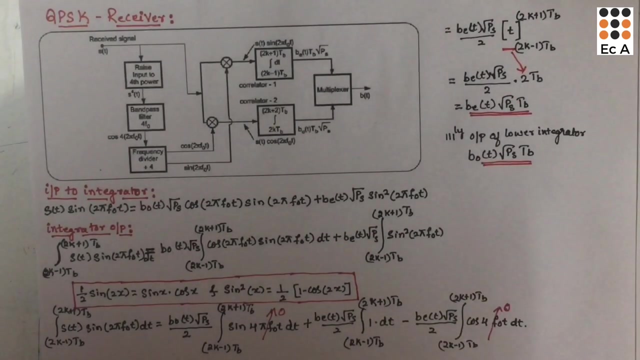 left out with be1 of t root pes divided by 2.. If we integrate 1, it is t between the limits 2k minus 1 tb to 2k plus 1 tb. So if we solve this we will get 2b. So we can write the above equation. 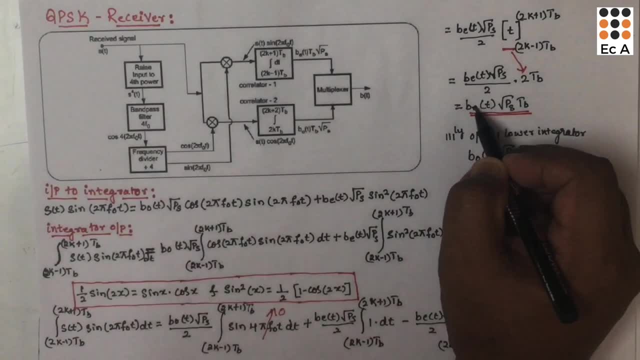 as be1 of t, root pes divided by 2 into 2 tb. So we can cancel out these two and finally we will get be1 of t into root PS, into TB. So this is the output of the upper integrator. So here you can see the output. 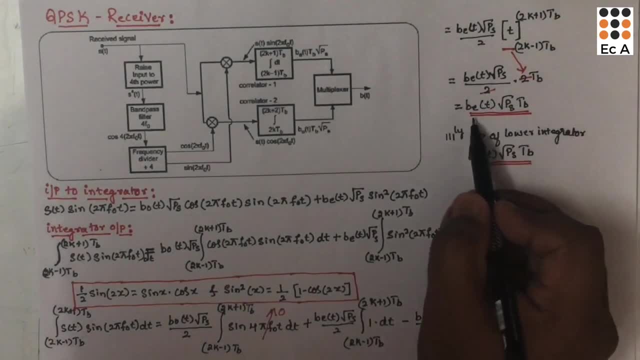 of the integrator is depending upon the transmitted bit, which is the even bit. Similarly, we can find the output of the lower integrator which we get as B0 of T, root, PS, TB. So this is the output of the lower integrator. Again, the output of lower integrator depend upon the transmitted bit, B0 of 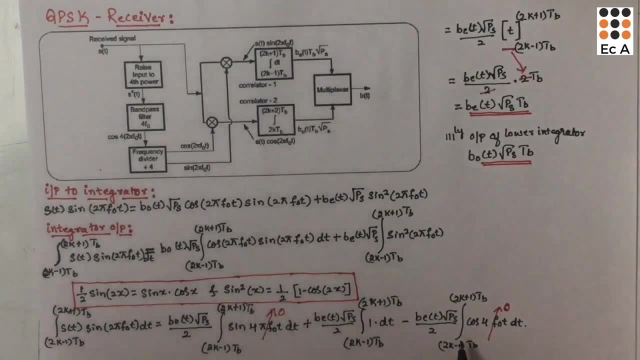 T. This is about the QPSK receiver. This is about the QPSK transmission and reception. Hope you have understood the topic. Thank you. 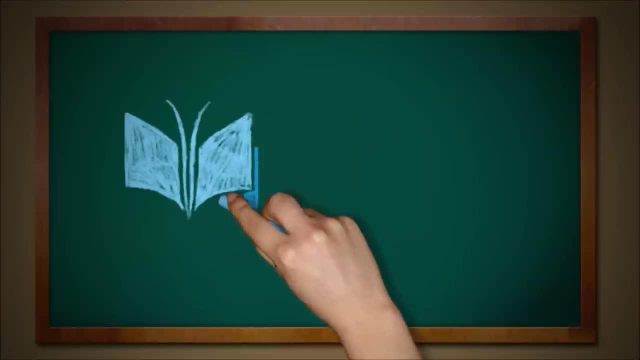 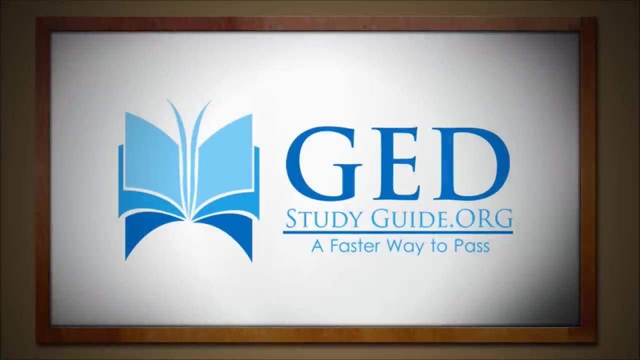 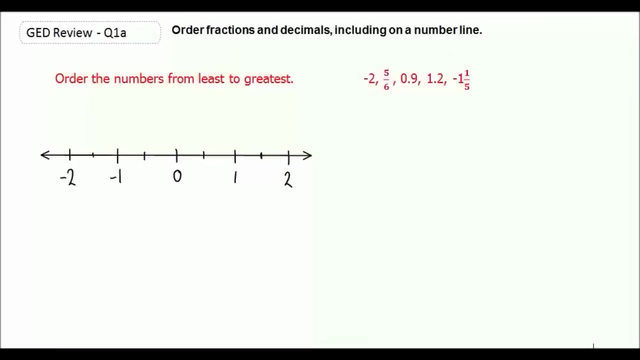 The first thing we're going to do is order numbers from least to greatest on a number line. We're ordering negative 2, 5, 6, 0.9, 1.2, and negative 1 and 1- 5th, So first negative. 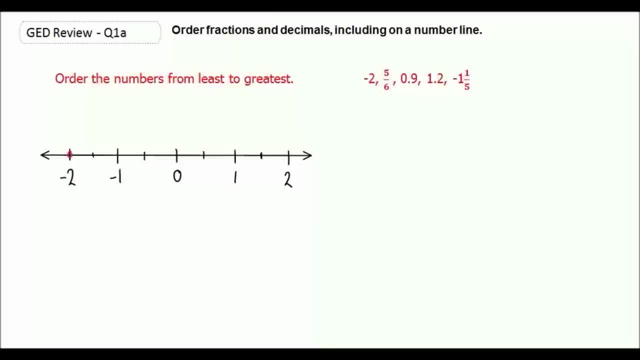 2, well, that's already on our number line, so we're going to put a dot there and just to remind ourselves we'll say negative 2.. 5, 6,- well, that's going to be a little bit more than 1 half and a little bit less than 1.. So 5, 6 would be somewhere around here.